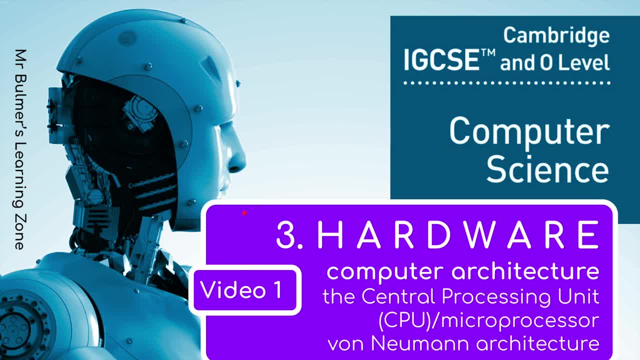 Okay, welcome back everybody. This is the first video for the third topic, the topic being hardware, to support the IGCSE computer science from Cambridge. We'll be covering the central processing unit, the CPU, the microprocessor, and we'll be looking at Von Neumann architecture in general. 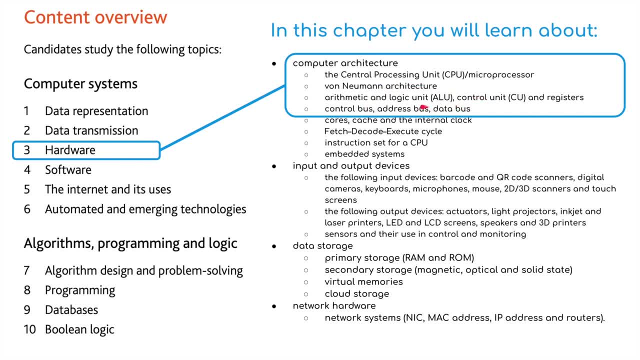 We will also look at the logic unit, the ALU, and the control unit and some of the registers. These are things inside of the CPU. We'll look at the control bus, the address bus and the data bus. This is part one of computer architecture. We will then move on and finish this in video two. 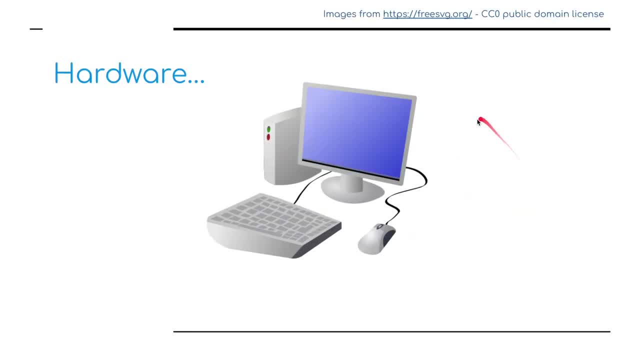 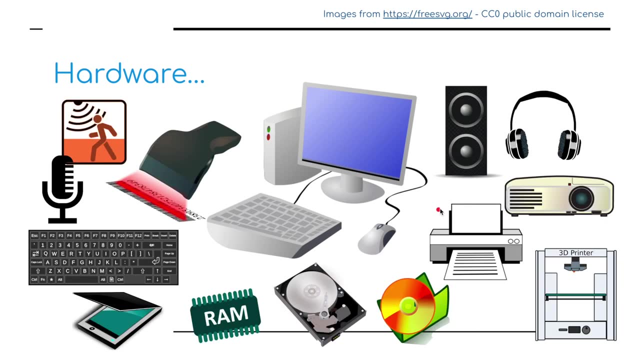 Okay, the topic is hardware. Hardware: everything that is sort of tangible, physical and digital On your computer, from the actual base unit itself, be it a laptop or a desktop computer- the monitor, input devices, sensors, barcode readers, your keyboard and your mouse, of course, output devices, speakers, headphones, projectors, laser printers, inkjet printers, 3D printers- to the things that are actually inside of the computer. 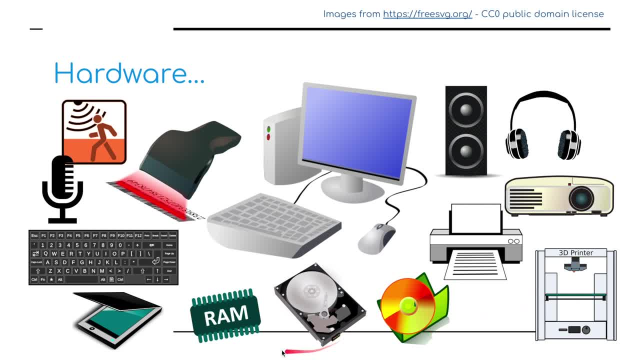 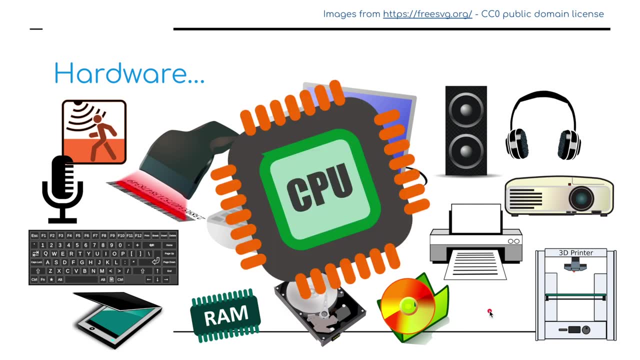 Such as the computer memory, the computer storage, and then external storage that can be sort of added to at a later date. So that's computer hardware. We're going to focus, though, on this thing: the CPU, the brains of the computer. 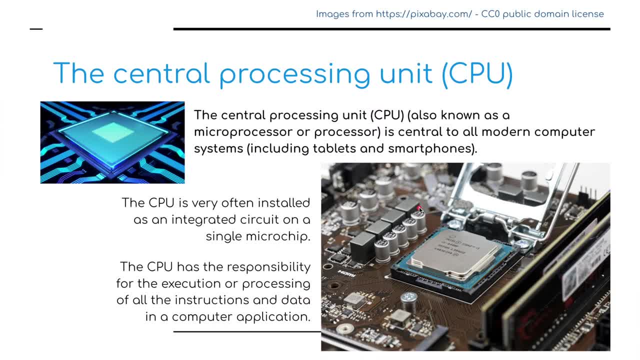 So here we go. The central processing unit, or the CPU as it's known, also known as a microprocessor or a processor, is central to all modern computer systems, Including your tablets, such as an iPad, and your smart phones. CPU is very often installed as an integrated circuit on a single microchip. 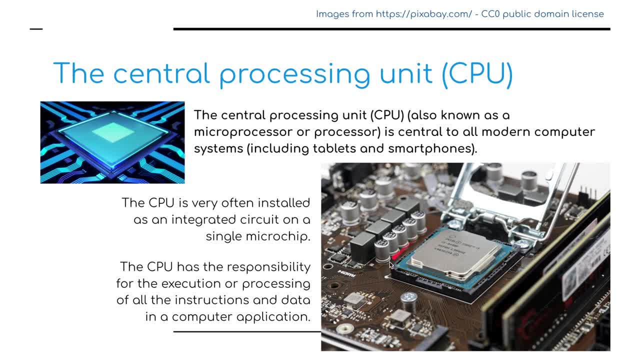 The CPU has the responsibility for the execution or processing of all the instructions and data in a computer application. It basically controls the input devices, the output devices, the storage, the memory, gets them all talking to each other and gets your computer doing specific jobs. 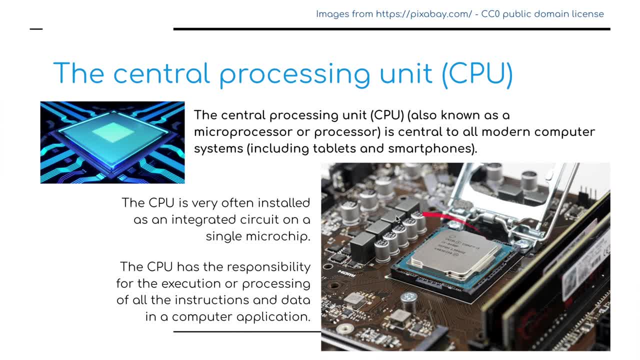 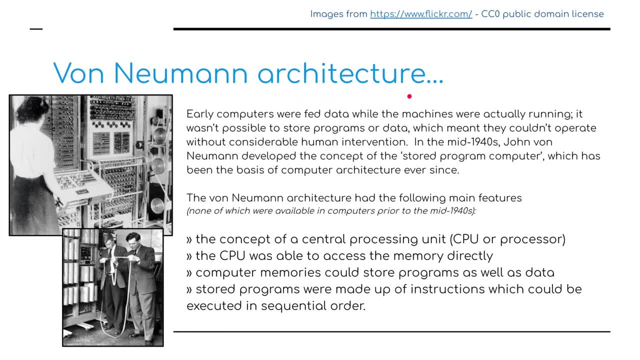 It is the brains, It's the central processing, It's the brains of the computer. So let's have a little look at the history behind computers and the chap called Von Neumann and Von Neumann architecture. Early computers, as we can see here, sort of turn of the 1940s. early computers were fed data while the machines were actually running. 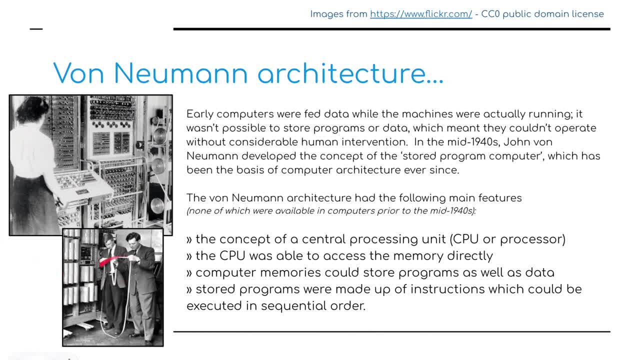 It wasn't possible to store programs or data, which meant they couldn't operate without considerable human interaction. Here's some guys getting ready, They're getting ready to feed off, looking at the results from this great, big, silly sized computer. In the mid 40s, John Von Neumann developed a concept of the stored program computer. 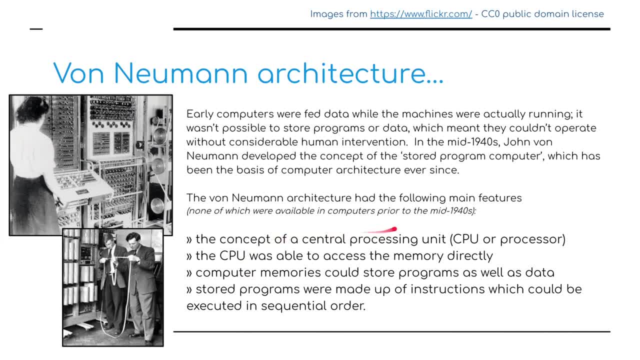 The stored program computer has been sort of the model for all computers ever since. So here we go. The Von Neumann architecture has the following main features: The concept of a central processing unit. Okay, It was able to access the memory directly. 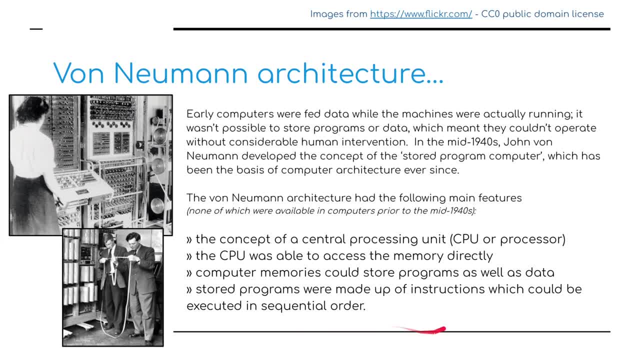 The computer memory could store programs as well as data, And stored programs were made up of instructions which could be executed in a sequential order. a program basically. So what is inside the CPU? Obviously, it's the brains of the computer, It's a central processing unit. 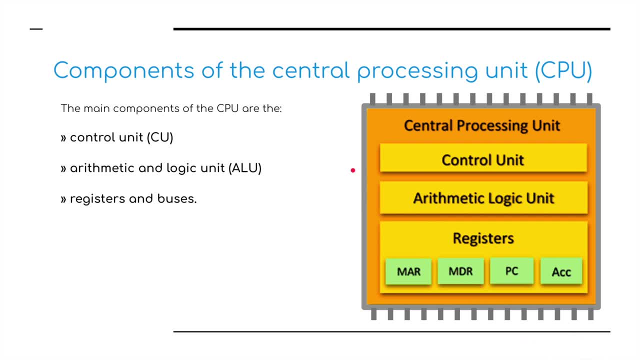 But what's inside it? Well, it's made up of sort of three distinct areas. Okay, We've got first of all the control unit, Then we've got the ALU, The arithmetic and logic unit, And then we've got a series of registers. 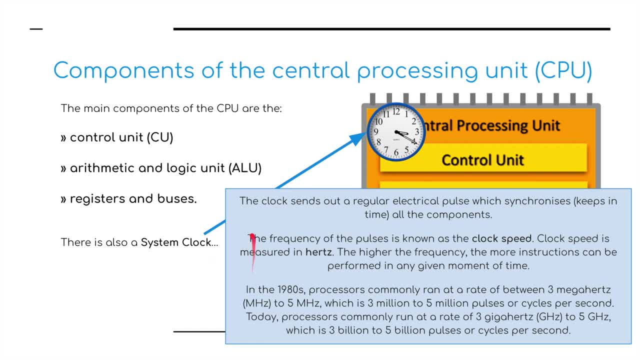 Okay. Also, and you'll be familiar with this, there is a system clock. Okay, This basically controls everything. It's like a timer which synchronizes all the components. It keeps them in time. Okay, Without this, the computer would simply not work. 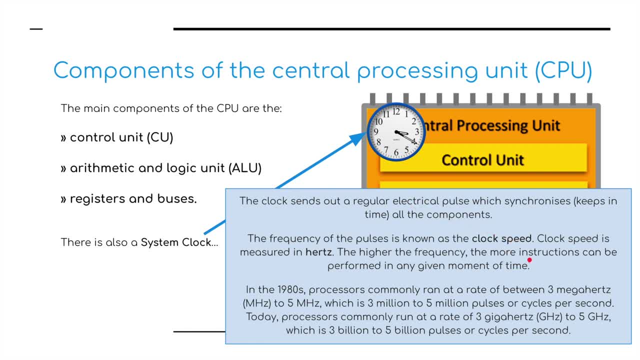 The frequency of the pulses is known as the clock speed. Clock speed is measured in hertz. The higher the frequency, the more instructions can be performed in any one given moment. In the 1980s, a little bit of history again. processes commonly ran at a rate between 3. 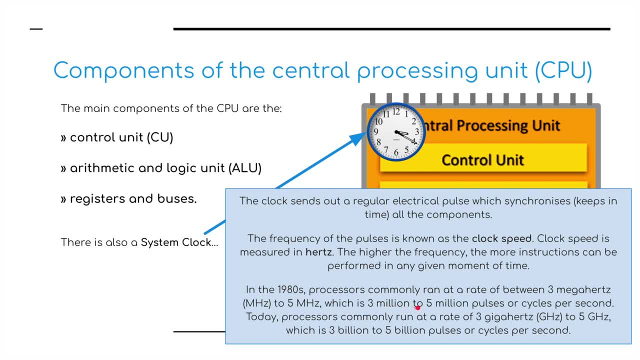 megahertz to 5 megahertz, 3 million to 5 million pulses or cycles per second. Now, in today's processes, these commonly run at anything between 3 gigahertz to 5 gigahertz, which is like 5 million to 5 billion pulses or cycles per second. 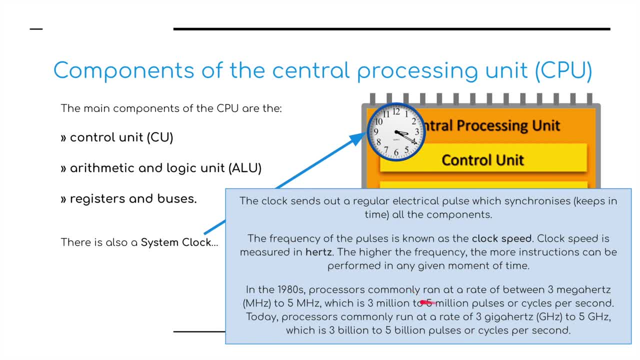 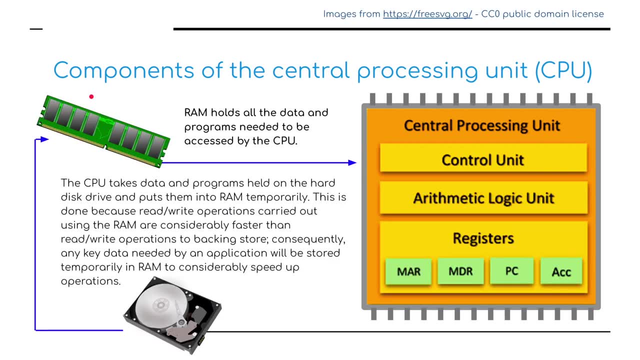 So you can see there's quite a jump from the 1980s to present day, sort of 40 years on. I just want to talk a little bit about what the computer's doing in terms of where it's getting its information from. 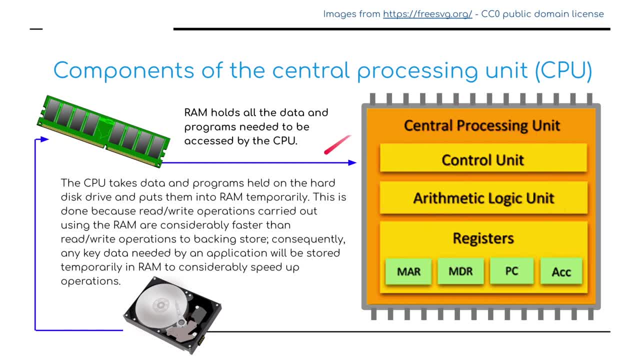 So the CPU takes data and programs held on the hard disk- this thing here- and puts them into the RAM temporarily. So I want to run something from Microsoft Word, so I'm going to find the program I've been working on on the hard disk. 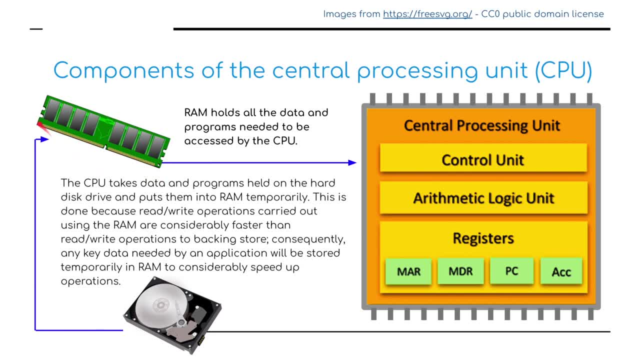 I'm going to load it into the RAM so I can work on it. This is done because read-write operations carried out using the RAM are considerably faster than read-write operations to the hard disk, to the backing store. Consequently, any key data needed by an application will be stored temporarily in RAM, to considerably 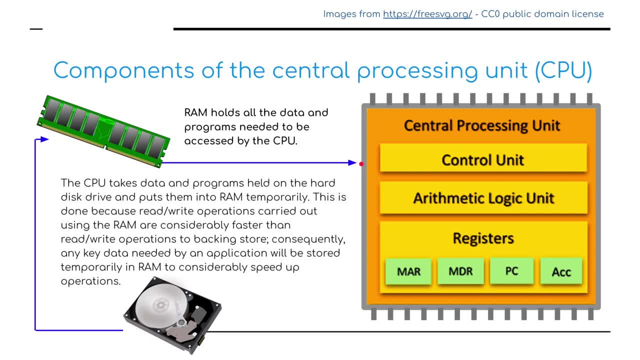 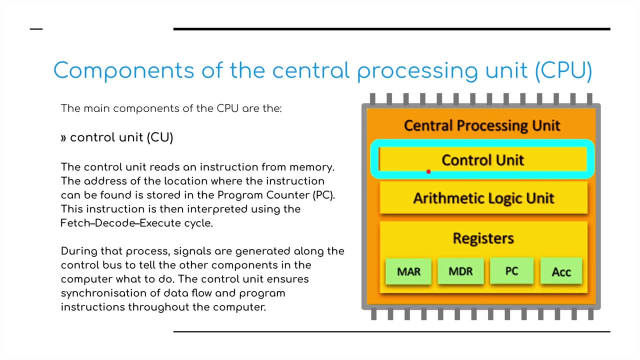 speed up the operations. So let's have a little talk about each of these. Each of these- Okay, Let's talk about each of these things, Starting with the control unit. The control unit reads an instruction from memory. The address of the location where the instruction can be found is stored in the PC. 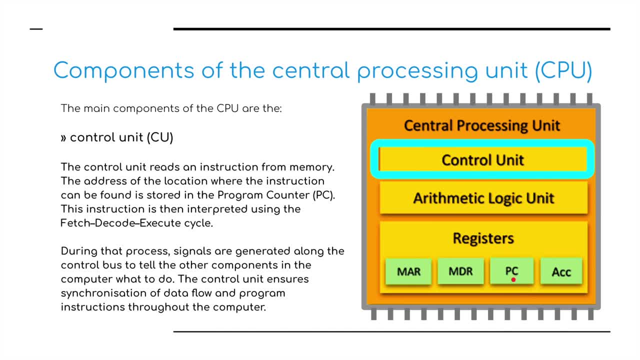 Yeah, the program counter register. This instruction is then interpreted using the fetch decode execute cycle, which we'll be covering in the second video. During that process, signals are generated along the control bus to tell the other components in the computer what to do. 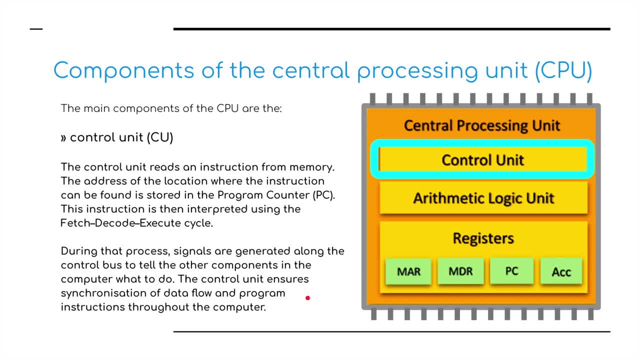 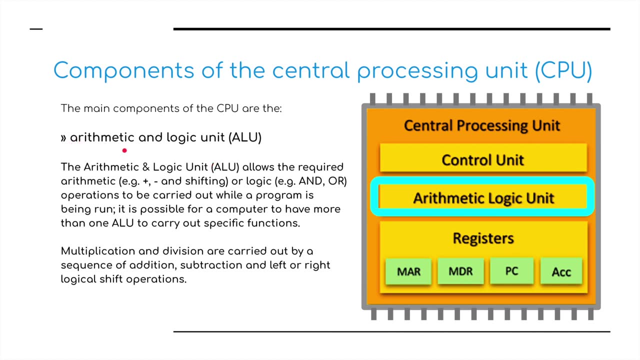 The control unit ensures synchronization of data flow and program instructions throughout the computer, controlling everything: The control unit. The next thing is the arithmetic and logic unit. As the name sort of suggests, this is used for mathematical calculations. It allows the required arithmetic or logic, basically pluses and minuses and shifting. 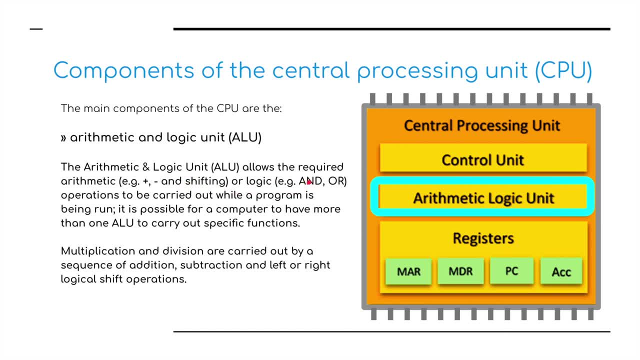 or multiplication and division, And the and and the, or basically the gate operations to be carried out whilst a program is being run. It is possible for a computer to have more than one ALU to carry out specific functions. As I just said, multiplication and division are carried out by a sequence of addition. 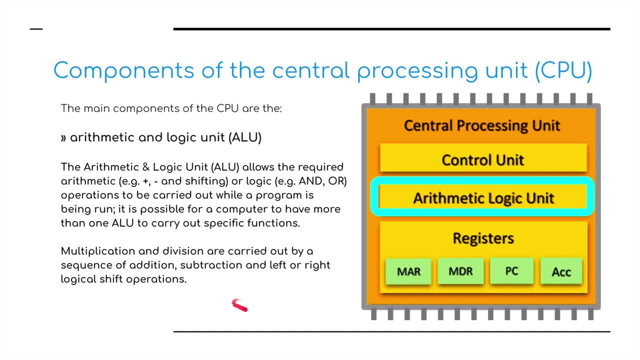 subtraction and left or right shifts. We have covered this in chapter one. Okay, Please refer to one of those videos if you want to talk a little bit more or see a little bit more about shifting. Okay, Up and down registers And finally, the registers. 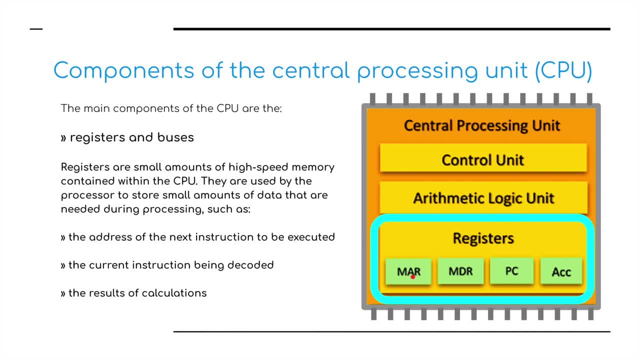 We have got the MAR, the memory address register, the MDR, the and finally, registers. We have got these four registers here which we will talk about a little bit later, But these are small amounts of high speed memory. These are contained again within the CPU. 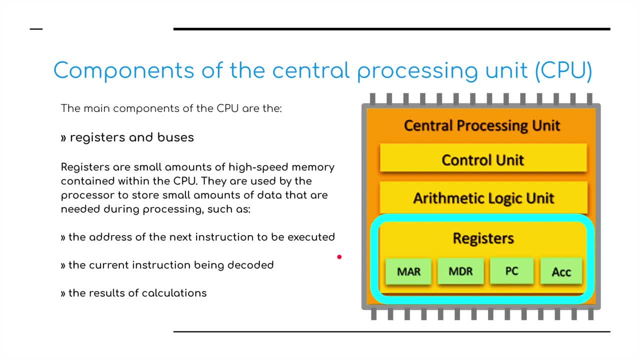 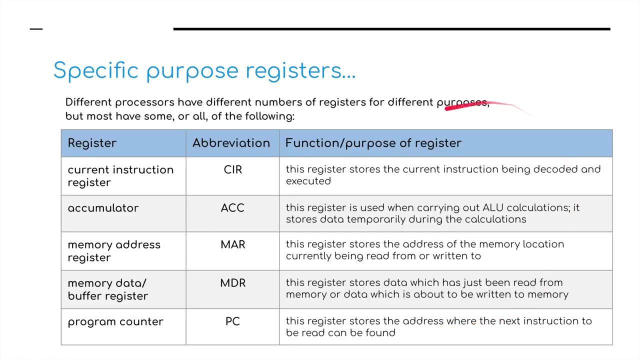 They are used by the processor to store small amounts of data that are needed during processing, such as the address of the next instruction to be executed, the current instruction being decoded and the results of calculations. Okay, And here is a little bit more of a breakdown of what these things do. 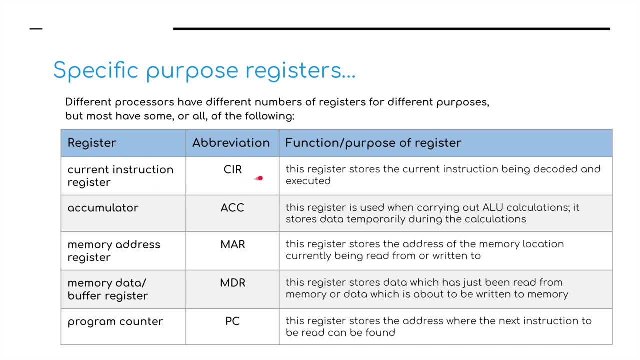 So we have the current instruction register, the CIR, We have got the accumulator, the ACC, the memory address register, MAR, Memory data or the buffer register, the MDR, and the program counter, And you can see what all of these do here. 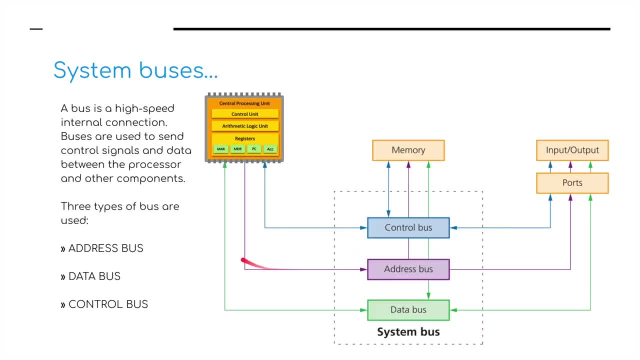 Okay, Moving on, How does the CPU talk to the memory And how does it talk to the input and output devices? Well, we use a thing called a series of things called buses. Three main types of buses: The control bus. 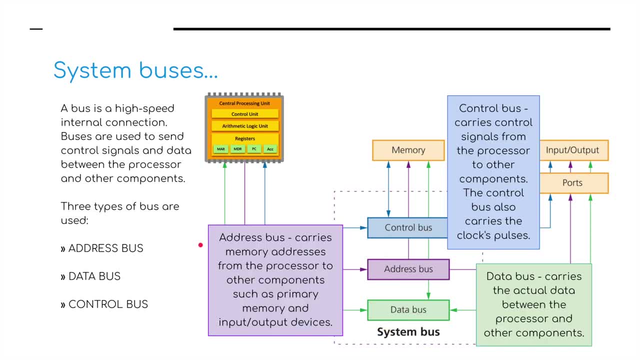 The address bus And the data bus. So, but what do they do? Well, the address bus carries memory addresses from the processor to other components, such as primary memory and input and output devices. The control bus carries control signals from the processors to other components. 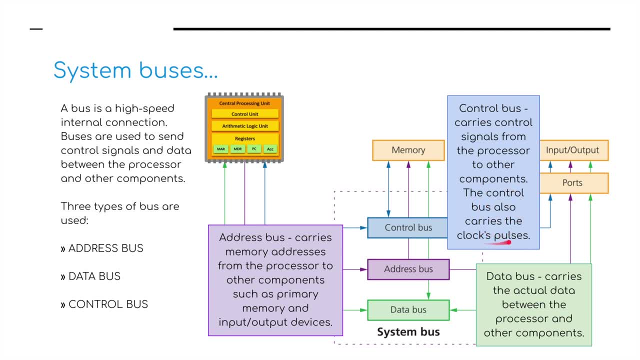 The control bus also carries the clock's pulses. And finally, the data bus. This carries the actual data between the processor and other components. Okay, So those three buses are carrying data, carrying information between the memory, the CPU and the input and output, or rather the ports to the input and output devices. 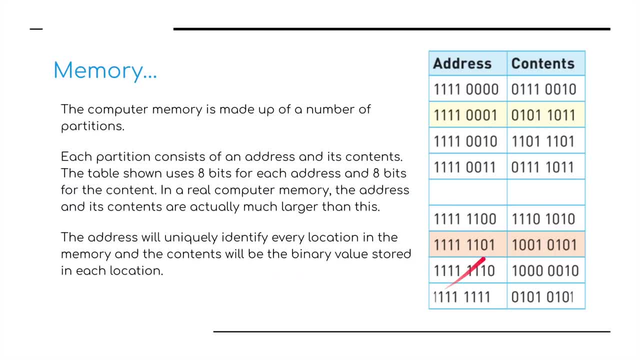 We will talk a little bit about memory, About where things live in memory. Basically, memory is made up of two partitions: The address, where something lives, And the content, Basically the information or the data. So the data and where it lives. 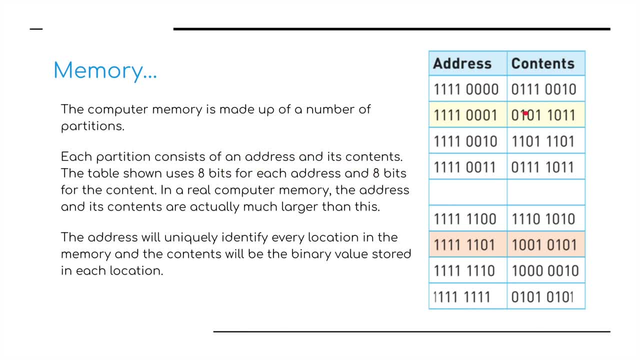 Each partition consists of an address and its contents. The table shown uses eight bits for each address. Okay, Eight bits And eight bits for the content. In a real computer, of course, the address and its contents are actually much, much larger. 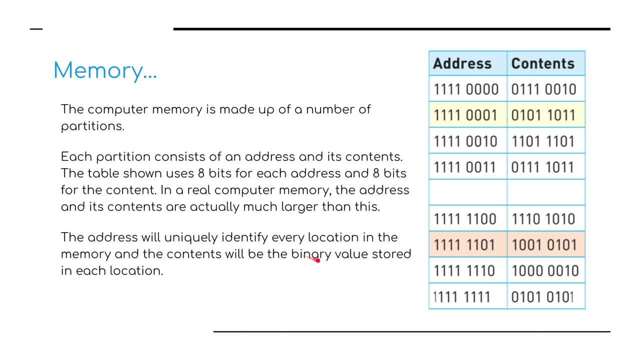 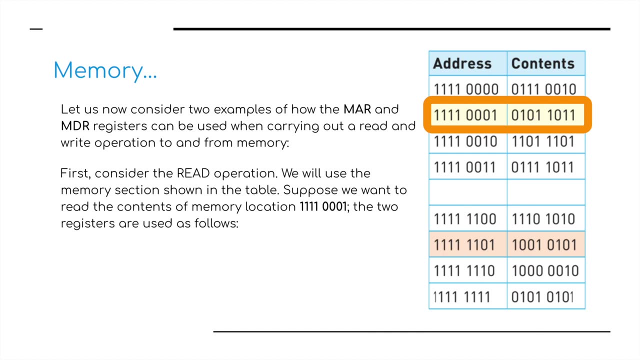 than this, The address will uniquely identify every location in the memory and the contents will be the value stored in each location. Okay, So let's talk about how information is retrieved and used from RAM in accordance with the registers on the CPU. So two examples of how the MAR and the MDR registers can be used when carrying out a. 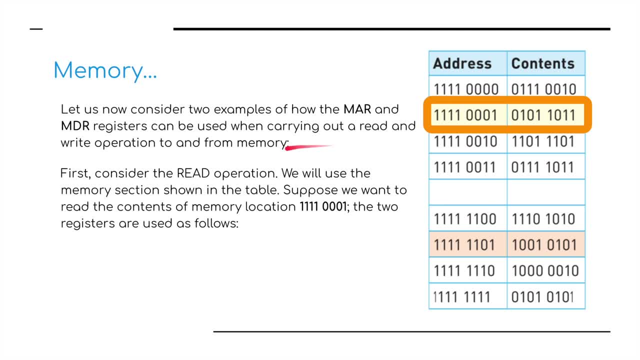 read and write operation to and from the memory. First, consider the read operation. Well, we will. Here we go. We've got a little address and content on the memory here from the RAM. Okay, Suppose we want to read the contents of the memory location. 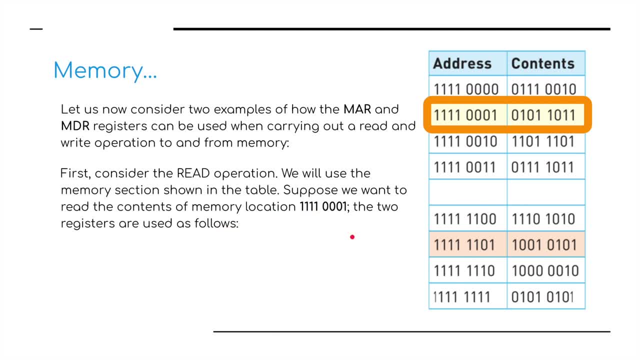 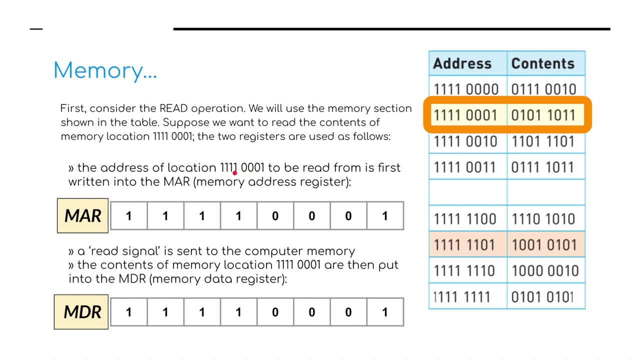 Yeah, The two registers are used as follows. Well, let's have a little look. First of all, the address of location 11110001, to be read from a list written into the MAR. So it writes this address into the MAR. 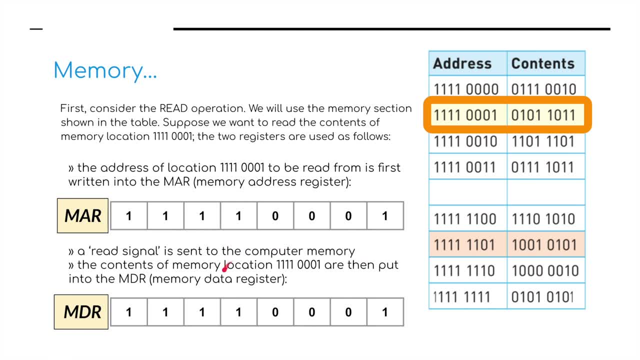 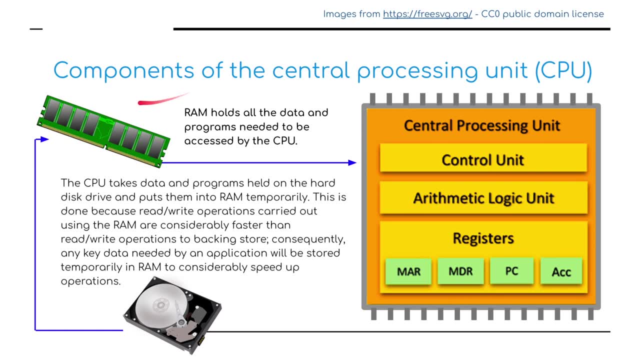 A read signal is sent to the computer's memory. The contents of this memory location are then put into the MDR. What is stored in this? Well, it's this data here. So two registers: the data and the address. Okay, 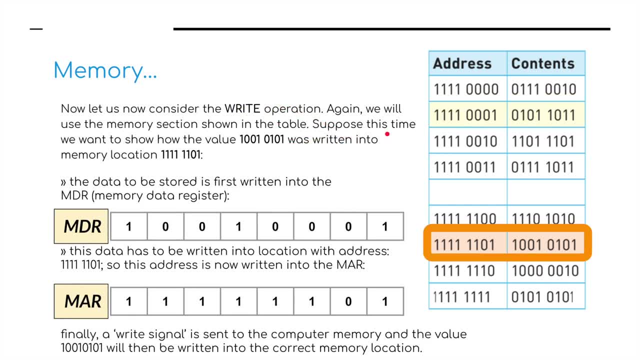 Now let's consider the write operation. Again, we will use memory section shown in this table, here, this particular section, here the one in orange. The data to be stored is first written into the MDR, the memory data register. Okay, 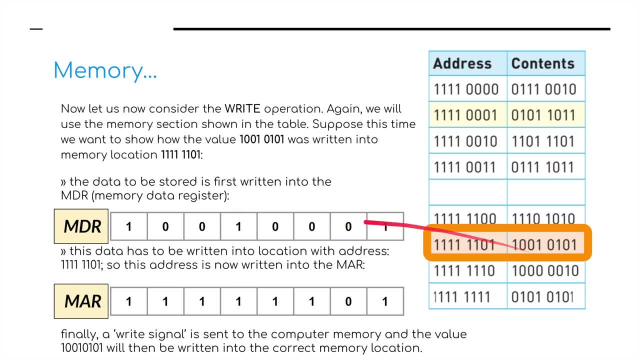 As you can see here we've put the data from here and we've put it into the MDR. So the content and the address on the RAM here, RAM memory- we've written it to the MDR on the CPU. This data is to be written into a location address here. 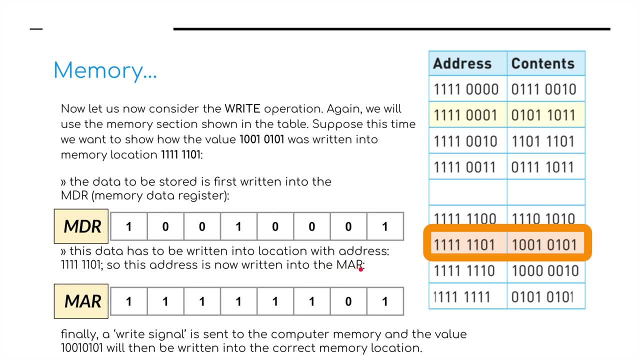 So this address is now written into the MAR. Okay, So we've put the address into the MAR. Finally, a write signal is sent to the computer memory and the value yep, this one here, will then be written into the correct memory location. 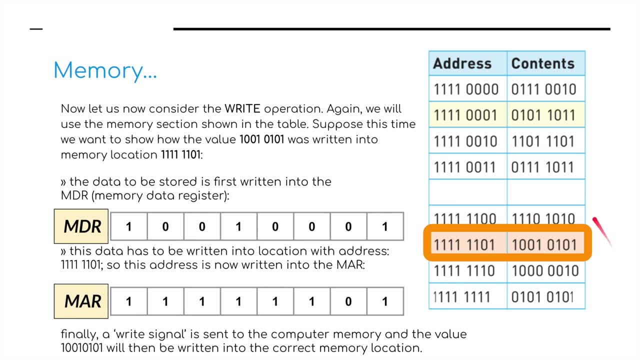 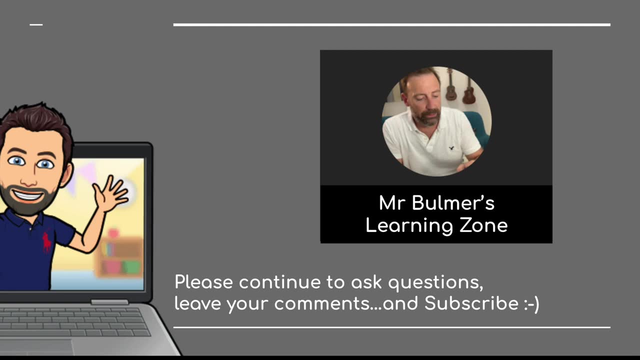 So that is it for memory. That is basically RAM, talking to the two registers, the MDR and the MAR on the CPU. That is it for this first lesson. As I said before, we will move on to the fetch, decode and execute cycle and finish off this first part. computer architecture. 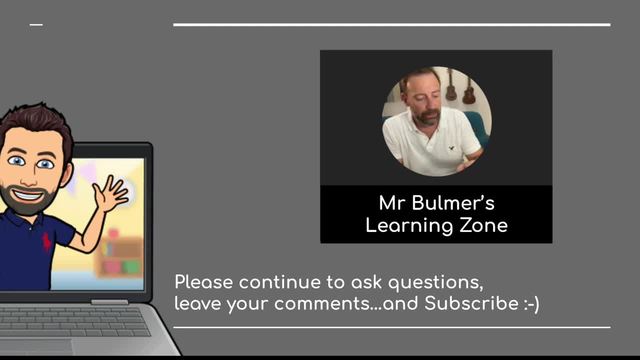 Okay, Thank you very much for watching. Please, please subscribe, if you haven't done so already, And I will see you very, very soon. Thank you very much indeed. 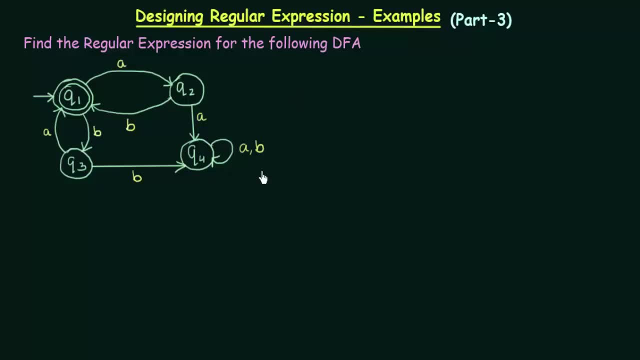 In this lecture we will be seeing another example of finding the regular expression for the given DFA. So here we have another DFA given and then we have to find the regular expression for this DFA. So here we see that we have states Q1, Q2, Q3 and Q4, where Q1 is the initial as well as the final state, and then we have inputs A and B.